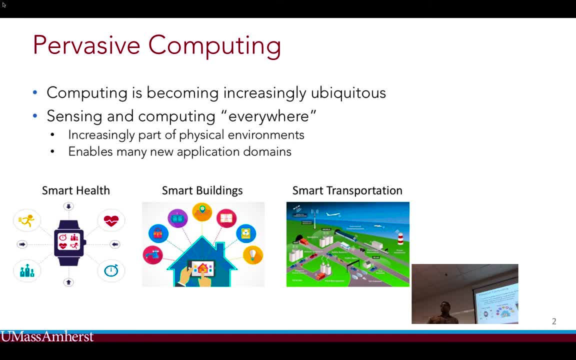 There is another concept called connected cars, where one car can communicate with another car, and that can lead to many energy efficiency benefits, which I'll be briefly talking about in a few minutes. So let's get started. So let's get started. 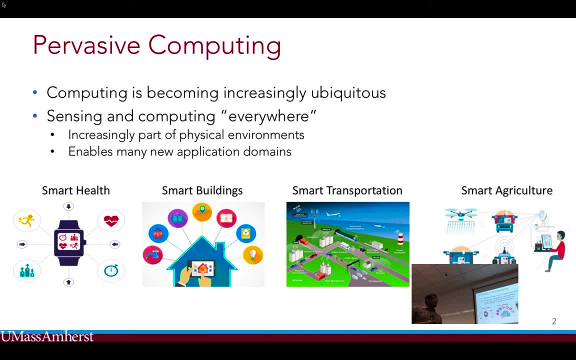 And finally, smart agriculture, where we have seen that people are using drones to monitor the moisture content of the soil On the ground, there are pH sensors which continuously monitor the health of the soil, And all these things can have led to increased yield. 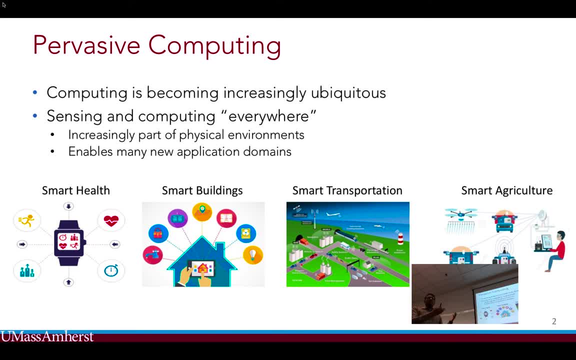 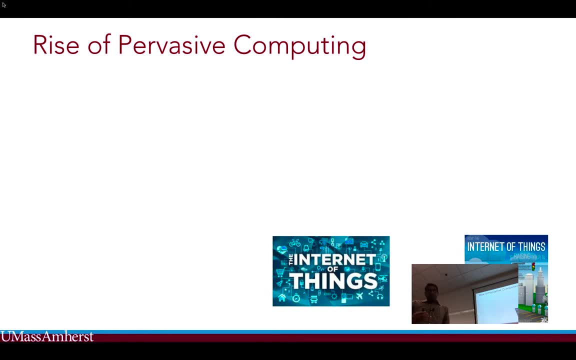 So there are significant benefits and we have already seen all these deployments part of our lives. Now there are couple of major drivers which have led to this rise in proliferation of pervasive computing. The first one is miniaturization of computing. So, for example, there are tiny sensors with computing and communication capability. 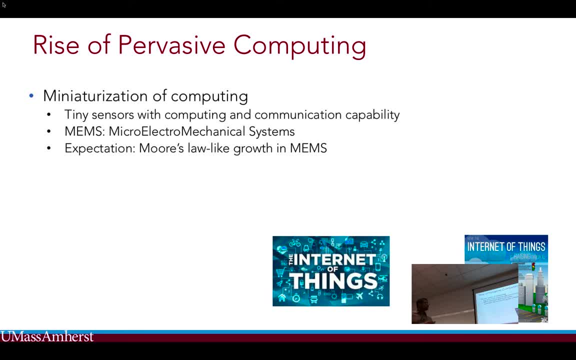 For example- you would have possibly- I don't know if you know this, but this term is often used- it's called MEMS, that is, Micro Electro Mechanical Systems. This is a slightly complicated name, but it essentially means that any sensor essentially 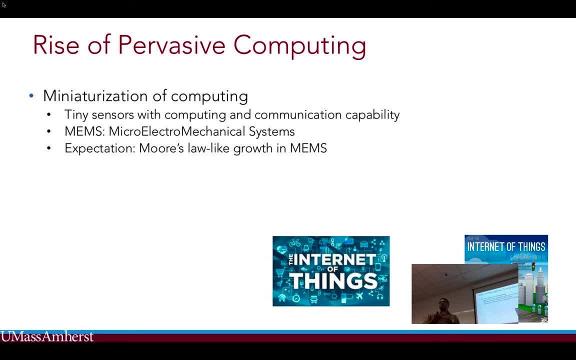 converts some kind of mechanical motion- piezoelectric effect, magnetic effect- into some form of electrical signal. Electrical signal can be change in voltage or change in current, And those and that change in current or voltage can then be further interpreted as recording. 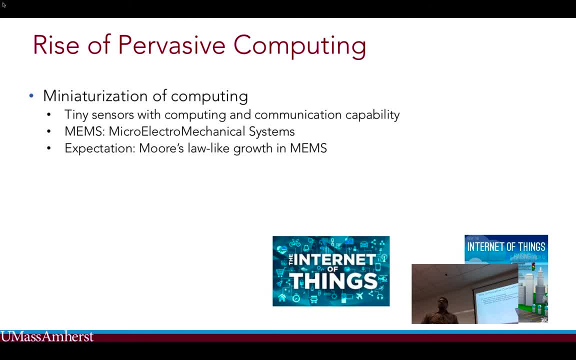 an amount of carbon monoxide in this room or some other measure And expectation is that in the future there'll be a Moore's law like growth in MEMS, in the sense it won't remain micro electromechanical systems, they'll become nano electromechanical. 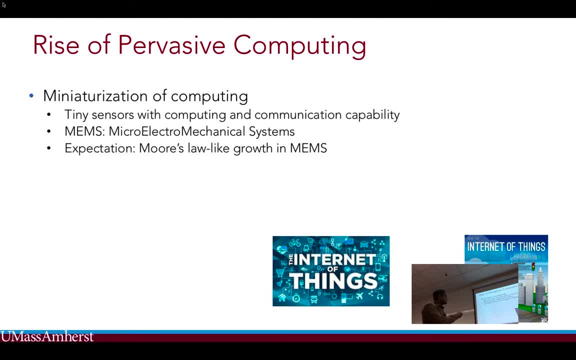 systems. So currently these sensors, which are classified as micro electromechanical systems, are in the range of 1 micron to 100 micron. This will There's orders of magnitude improvement in the size of these sensors, And also we have all heard this buzz term called IoT, this Internet of Things. 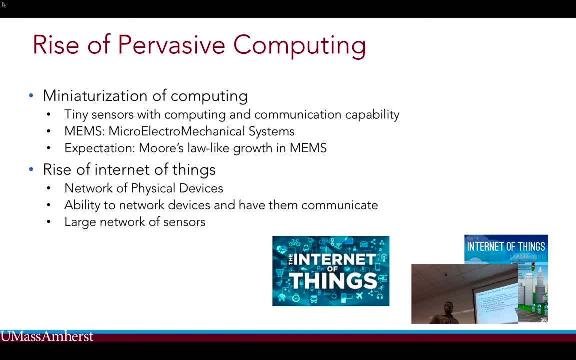 This essentially means that all our physical devices now have the capability of exchanging messages among each other. For example, occupancy sensor can convey message to a Nest thermostat that there's nobody in the home. Possibly we can turn off the air conditioning unit, And there are many other applications. 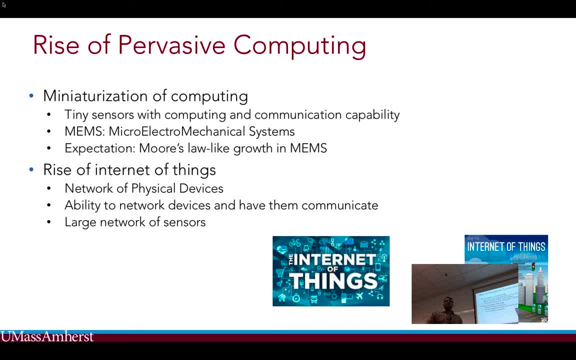 Which involve more than just two devices communicating. Any modern industrial plant will have thousands of sensors which are communicating with each other through what they call machine-to-machine communication. They might use some low-power communication systems such as Bluetooth or ZigBee. There are different protocols. 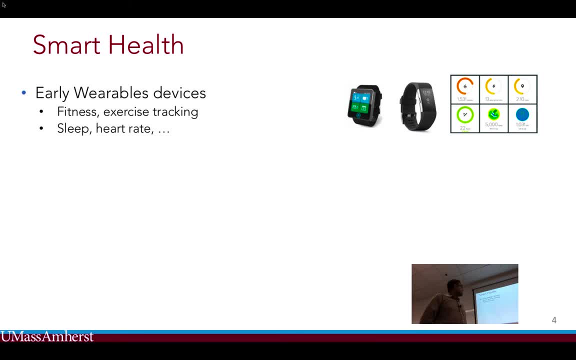 And now let me focus on one of the important applications, And that is the Internet of Things. The Internet of Things: The Internet of Things: Communications and interaction. The Internet of Things. Content creation was huge on Windows and Ferrinte and Ubuntu. 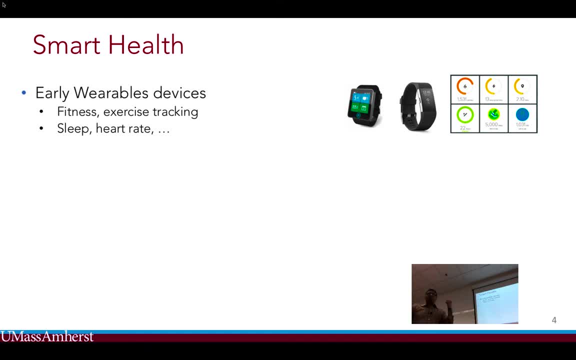 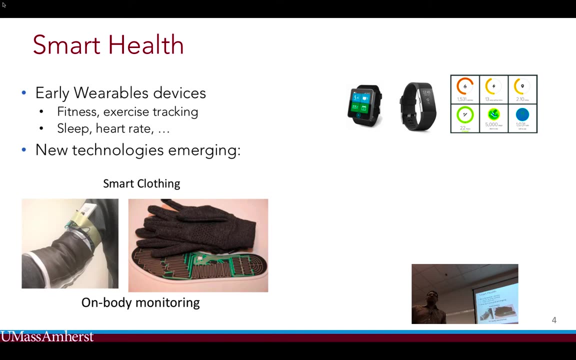 Theord was, In fact, the Cutter of Civilization, was huge In terms of the Internet of Things. it's like I said before: there is no internet of things. space, you're the π, that's the theorem You're saying. You're saying goodbye to the Internet of Things. 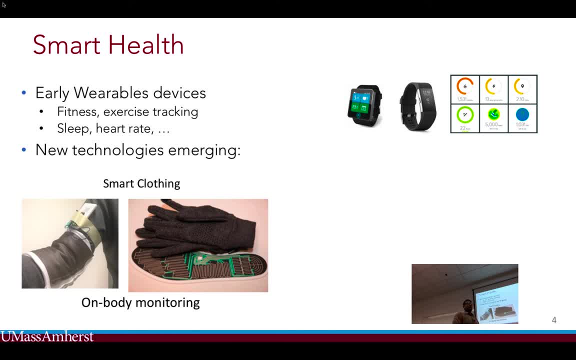 Absolutely Retrieving the device. Hey, what do you mean? here's just a piece of paper, but for me it is bit invasive and maybe this is not for everyone. So imagine your clothes that you're wearing already recording all this information, which are already tracked by. 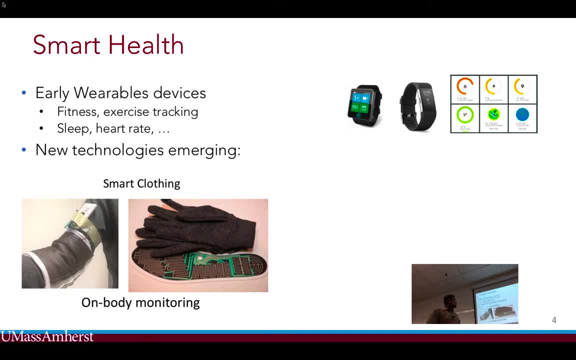 these variables, and this is already happening right now. So there are these smart gloves or smart shoes. They can also use to detect sweat, which is used to detect anxiety in some drug addicts and also normal people who are working in an IT environment. So there are a lot of cool applications of all these sensors. 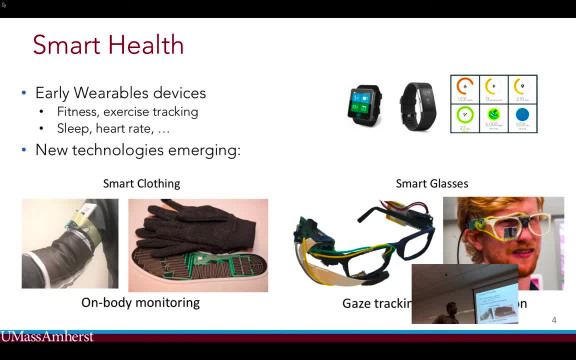 Also, in fact, in UMass itself, we have this project called Smart Glasses, where you can have this glass thing, spectacle, which is equipped with a camera and that can actually track the gaze. that is how your eyes are moving while watching a computer screen. 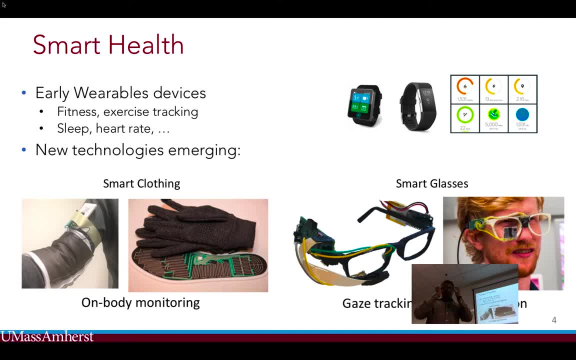 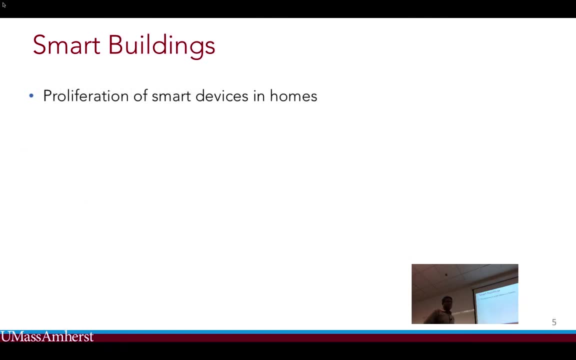 and this is used in fatigue detection. Also, there is, I think, a contact lens from Apple which can detect your blood sugar level. So there are quite a few applications of smart health When it comes to buildings. currently, all buildings are filled with lot of smart devices. 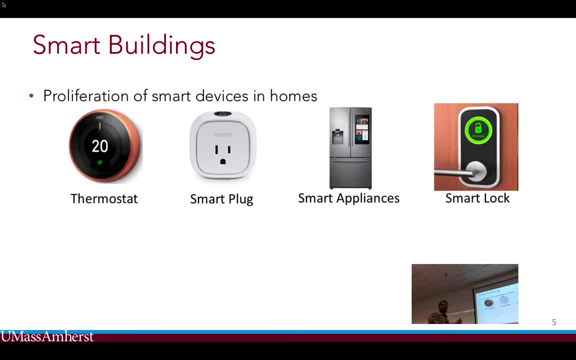 I already talked about the Nest thermostat, which is what Nest calls a learning thermostat. It can look at past occupancy pattern and learn a schedule of when you leave the house, when you sleep, and basically then it can control your ACs or heaters so that the living 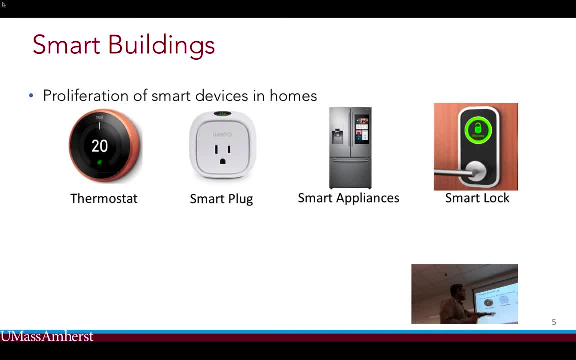 environment is very comfortable. Also, there are these smart plugs, So these are at plug level. you can measure the energy consumed by refrigeration, refrigerators, washing machines, different appliances that are present in your house, And also you have these smart fridges, which can actually maintain a 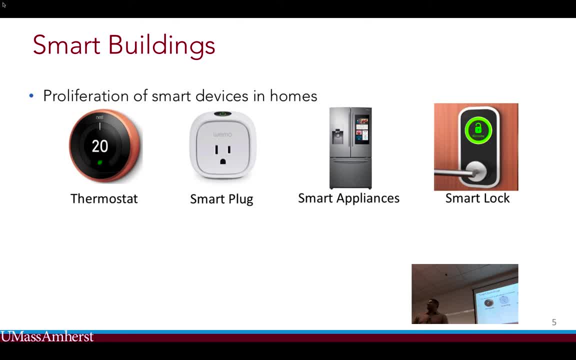 grocery list of items that you may need to buy. The current smart fridges are not necessarily that smart. You have to enter all that information. Essentially it's a tablet on a refrigerator, but in the future it is anticipated that they can actually detect food spoilage through some sensors, because when food spoils, 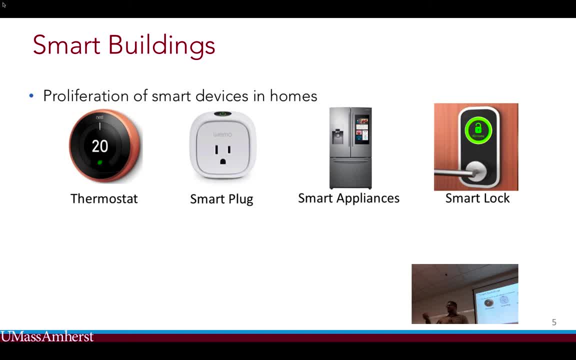 they release some kind of ammonia or some gas at a very minor level. Maybe those sensors will be installed in the future. They can possibly look at expiry date of your food and send you an alarm that possibly you need to get fresh milk because the milk is going to get spoiled. And also there is something 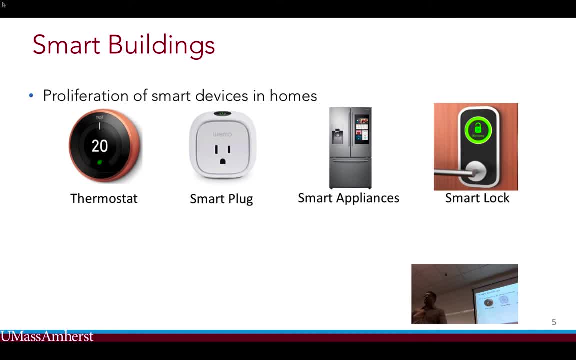 called as a smart block. So essentially you can open your door with the help of an app And increasingly all these smart devices are controlled through phone or voice interface. I don't need to go into detail of these things. You know that there is. 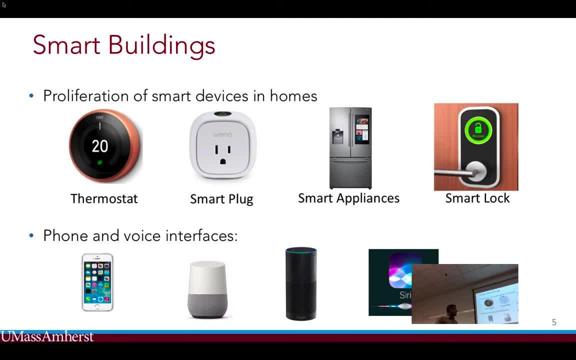 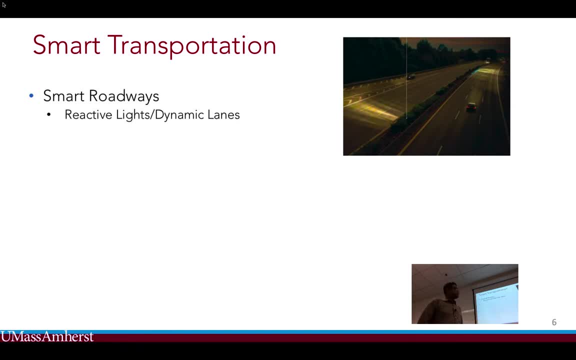 Alexa Siri app in most of the iPhones. Now let me go into another application domain, that is, smart transportation. In front of your screen, there is this picture of reactive lights being installed. So, based on the proximity of a car which might be going on this road, the sensors on the road can detect the motion of the car. 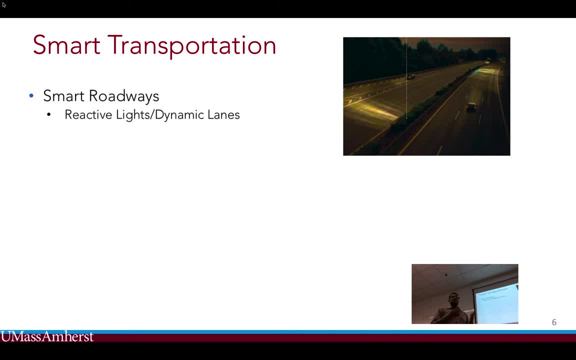 and automatically turn on the lights, So this can result in saving a lot of energy. instead of having street lights that are always on, With this system, you can actually save a lot of energy. Also, you can have dynamic lanes. So imagine, instead of a physical line which separates one lane to the other, there are these. 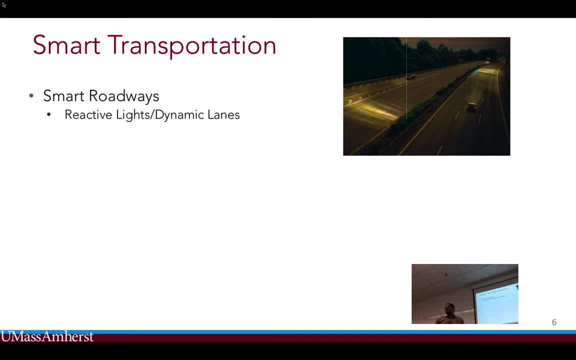 lighting lanes which can possibly, if there is any repair activity happening on the road, these can lead travelers to go take the right path. Similarly, road condition can be monitored and there can be traffic management solutions. So in the city of Austin they have installed. 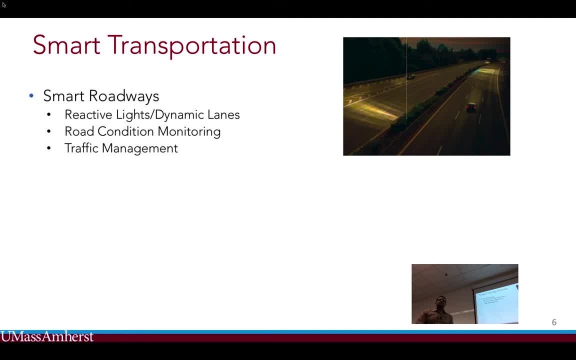 around 170 Bluetooth beacons, and every time a road crosses that cross section, your MAC ID is essentially noted in their databases, and when you again cross some another cross section, they can actually calculate the amount of time you took to travel between these two points. So 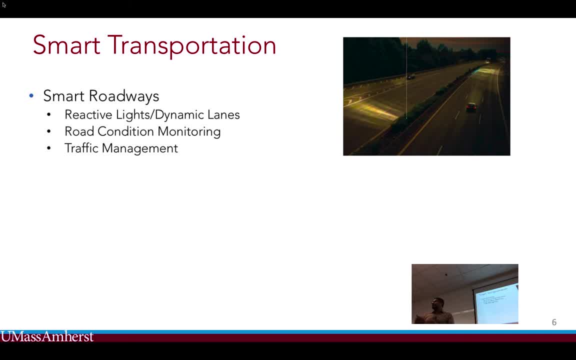 you don't have to monitor each and every car. If you can just monitor a few cars which have their Bluetooth devices on, they can essentially make a good estimate of the amount of traffic that's on the roads, And they can dynamically change the traffic lights to make sure that there is no congestion in our roads. And this 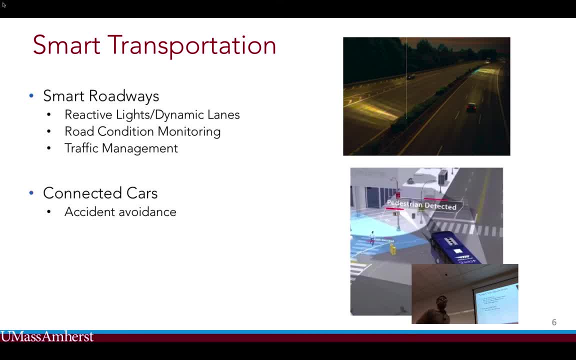 is already happening, So these are not paired. If it notices that there is a Bluetooth device that is on, even then the MAC IDs can be registered. You don't need to pair. essentially You need to pair to transfer data or send some kind. 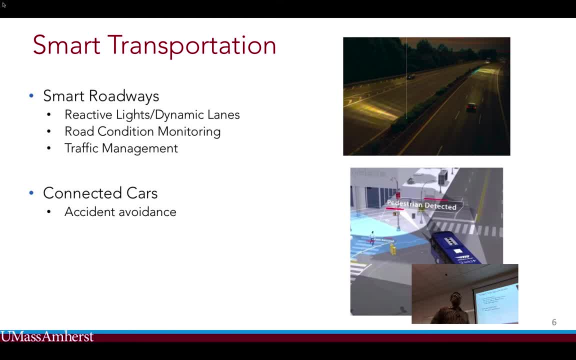 of signal. okay, turn on my headphone, or something like that, But isn't this invasion of privacy? Oh yeah, so the whole lecture today is about invasion of privacy and I'll possibly not venture into that, because I am not the right person to answer these questions. I have not. 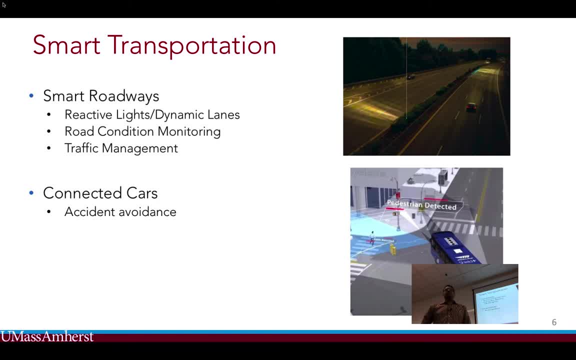 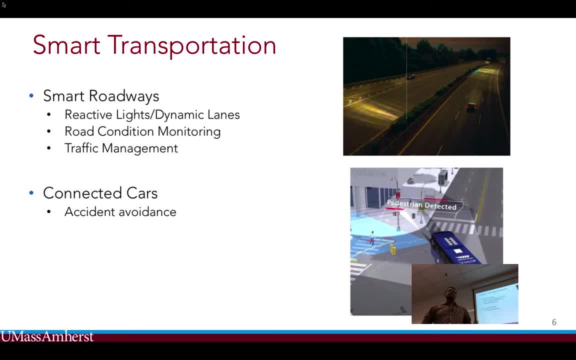 There needs to be a discussion- I mean not just among computer scientists, but also the policymakers, governments and also individuals- to decide how much they want to share and how much they are comfortable with. So I'm very sure the city of Austin didn't take a poll saying that, okay, should we install? 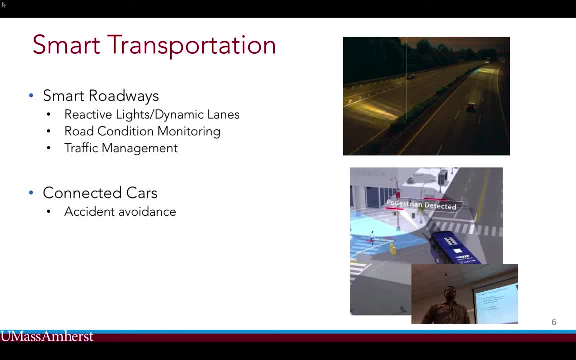 these Bluetooth sensors everywhere. But yeah, it's a very tricky question. actually, Part of it is a computer science problem to set up right policies So that users have access to their data. Part of it is the soft side of things You need. 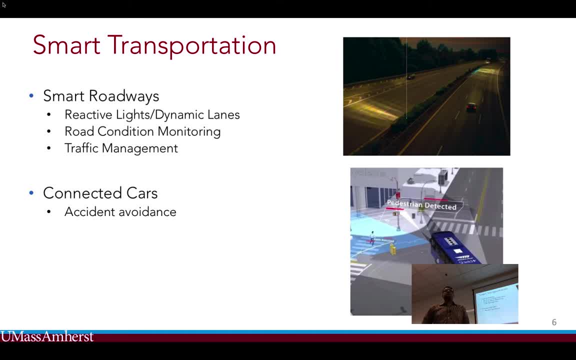 more discussion on it Probably involves some social scientists. to answer that question, Yes, so connected cars is another cool application. So, apart from the basic use case of accident avoidance through detecting pedestrians, So one bus car can be used to detect pedestrians. One bus can say that, okay, there's a pedestrian walking and it can inform some another car. 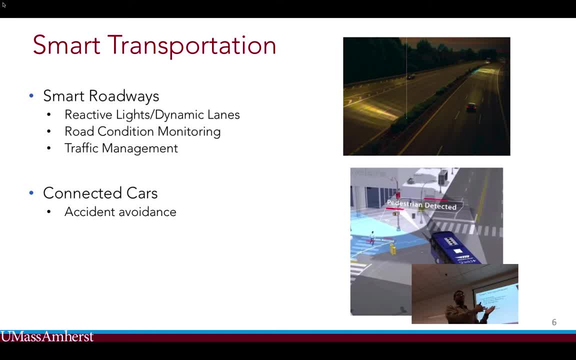 which is behind it, But that car may not directly see the pedestrian. So those are the use cases where connected cars will come into picture And this has implications in fleet management. So there are lots of trucks carrying cargo all across the country, all over the world. 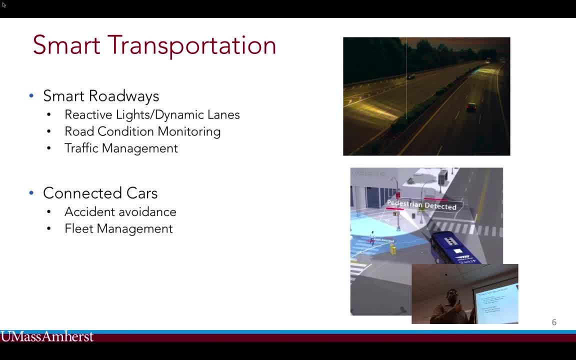 in fact, And imagine these trucks communicating with each other, their speed, their traffic conditions, So they can actually travel much closer to each other. because it's safer, They can be controlled. possibly even the brakes can be controlled by these sensors, And that can. 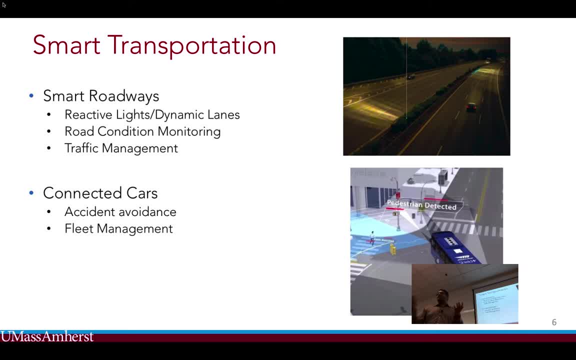 save a lot of energy in terms of. you would have seen in every traffic signal. So the first car moves and the last car takes some time to move. With the connected car, all the cars can start at the same time, rather than the delay getting propagated All the. 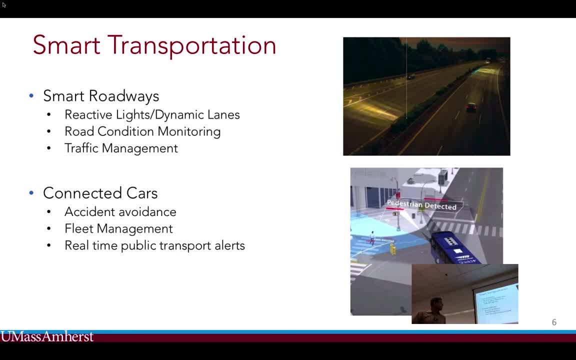 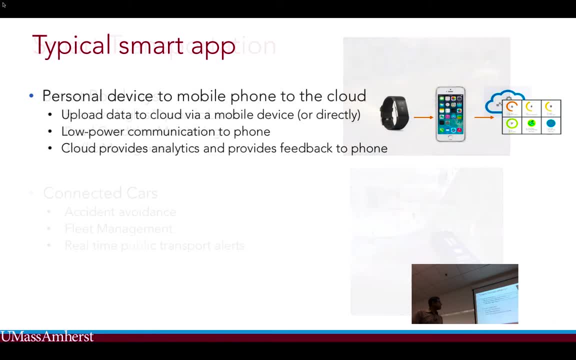 cars will start at the same time or stop at the same time And of course, even connected cars can be used in real-time public transport alerts. Now I mean, we have seen a lot of cool application domains, but how would one go about building? 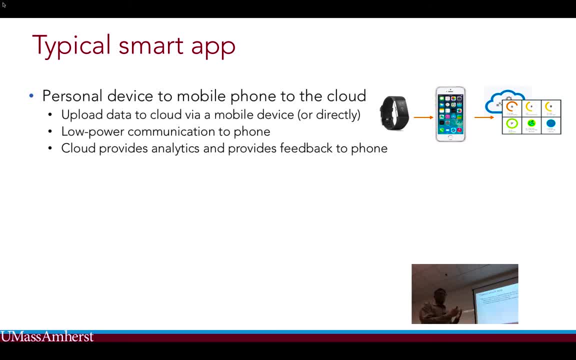 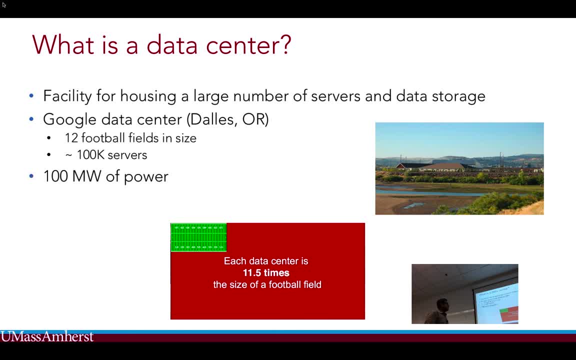 want to communicate with the cloud. You want to communicate with the cloud. You want to communicate 100,000 servers, and the power consumption at its peak capacity is around 100 megawatts of energy, So that's enough to power a small city. 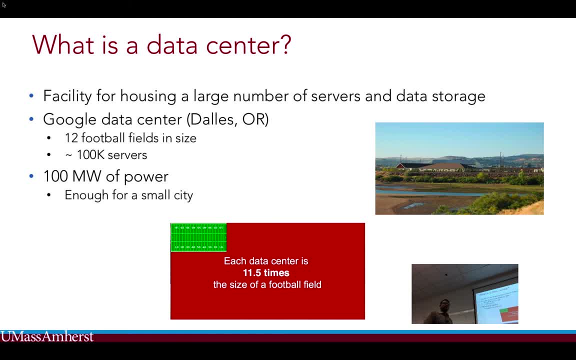 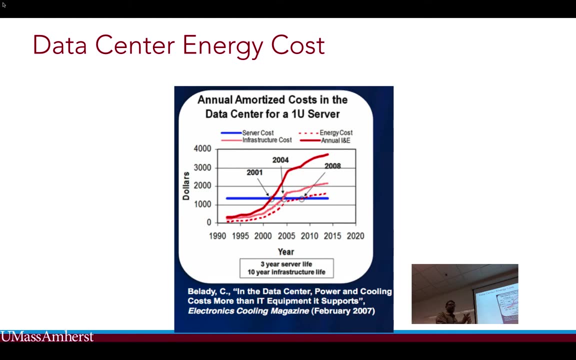 Now, obviously, Google doesn't want to spend that much energy. They want to make sure that you save money and improve your operations. So this is an important problem and they are heavily interested in this one. So, before going into the scale of 100,000 servers, let's look at the cost of one server. 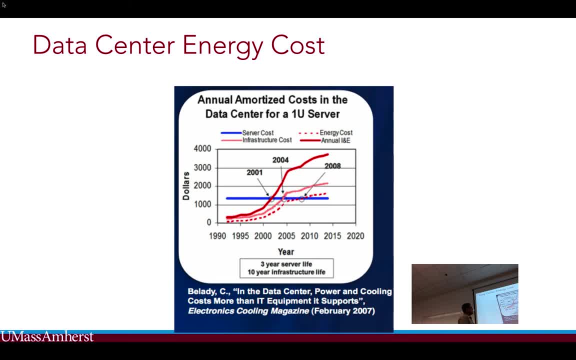 in a data center. So in this graph the blue line actually shows the cost of a server, that is, cost of buying a server. considering a server, life is three years, So they have assumed a high-end server of $4,000 and IU is essentially a unit of rack. 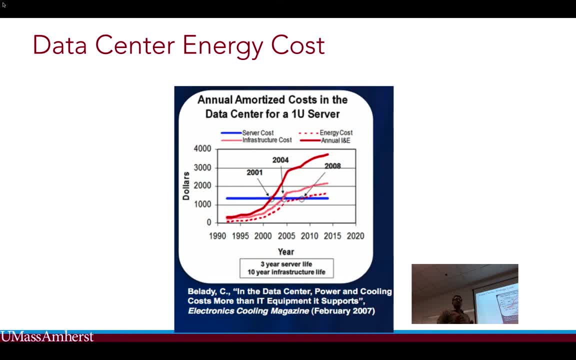 size. So IU means 1.75 inches. So a server of that size which will fill that much space in a rack, in a data center. And, as you notice, the cost of the server has not necessarily increased or decreased with time. So that's an immediate observation. 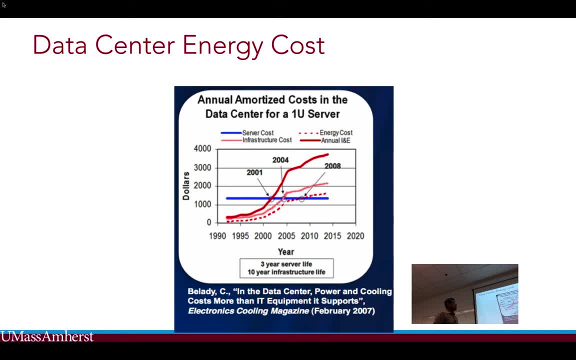 But there are two other costs involved here. One is the energy consumed by these servers, which is increasing. with the energy costs are going up, The energy bill of the servers will also go up. And the second cost is the infrastructure cost, that is, to cool the infrastructure. 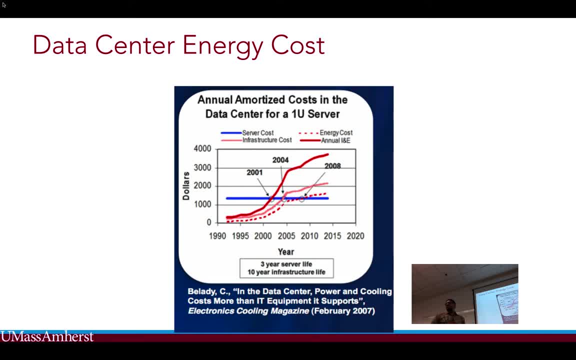 So all these data centers have massive cooling needs. The heat has to be taken out of these data centers, So a lot of energy is used in maintaining the temperatures of the data centers. So all this cost is actually higher than the cost of the server itself, which is not ideal. 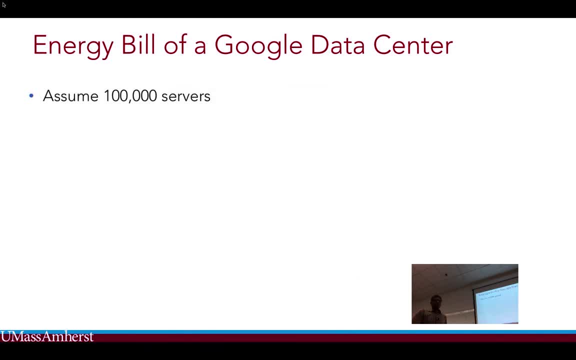 Now we can focus on the Google data center that we discussed earlier and let's see what's the energy cost involved in this data center. So, as I mentioned, there are 100,000 servers. Monthly cost of one server is around, say, 500. 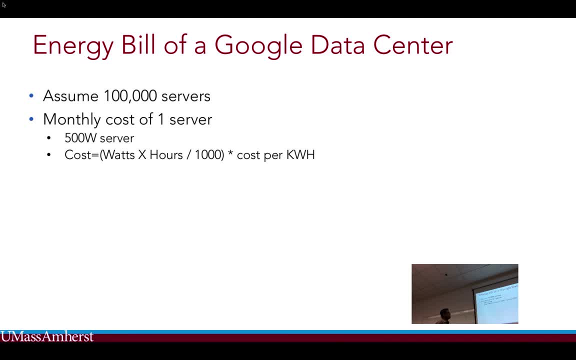 The power consumption is 500 watts. So if you want to calculate the monthly energy cost, it's around $50.. Now multiply that by 100,000. That's about $50. That's about $50. That's about $50.. 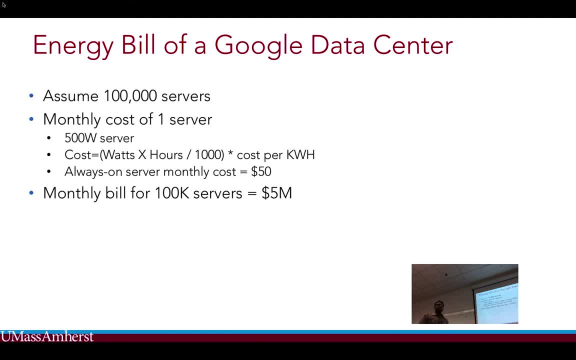 So if there are 100,000 servers, if they're always on, the number comes to $5 million. And what's the cost of cooling then? So people in the industry who work with data centers use this term called PUE, That is the power usage efficiency. 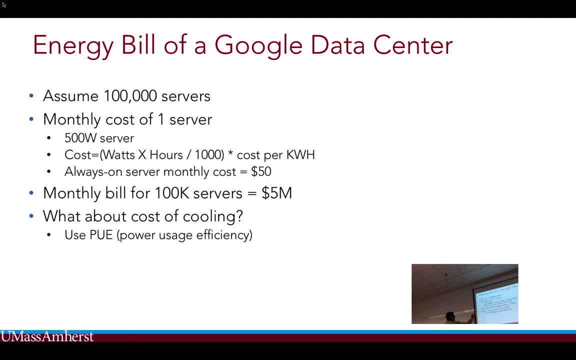 So power usage efficiency is nothing but the total energy cost divided by the server energy energy cost. So if cooling requires five million dollars and the monthly bill of running a service five million dollars, then the PUE is around two. That is server cost plus cooling cost divided by the server cost. But Google data centers 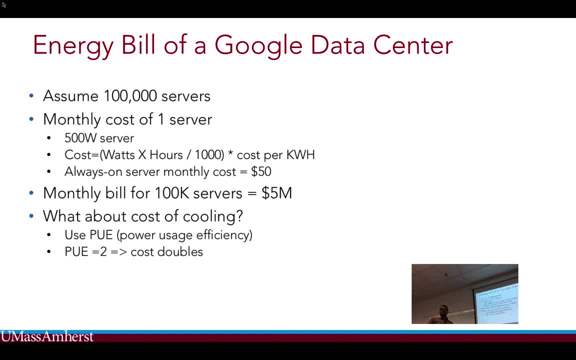 are pretty efficient. They have designed their complexes in such a way that the heat is taken out quickly. They have housed their data centers in colder climates so you get free air from outside, free cold air from outside. So the Google PUE is around 1.2.. That is the cooling cost is 20% of running the server cost. It's just. 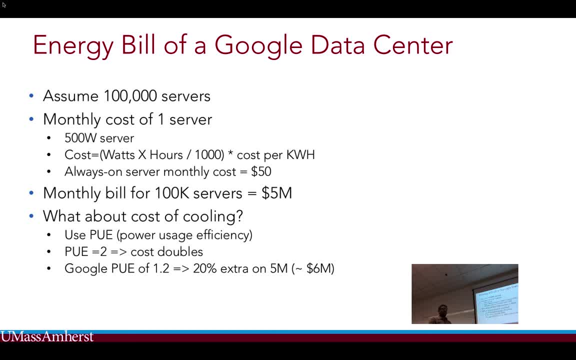 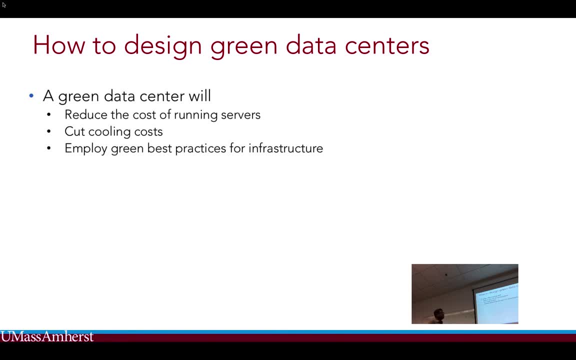 a number that we need to consider. It's highly efficient data center. Now, designing an efficient data center involves following things like reducing the cost of running the servers. cutting cooling cost. employ green best practices. Now let's look at each one of them. So reducing server cost can. 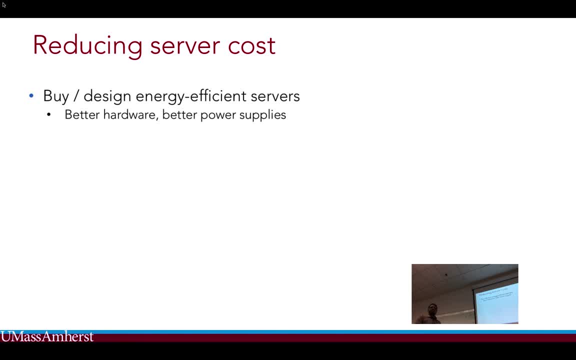 be done in different ways. One thing is to employ better hardware. Newer and more efficient CPUs are entering market at an increasing rate, So the cost involved, the computations per watt, is improving, So newer machines obviously would spend less amount of energy. There are better 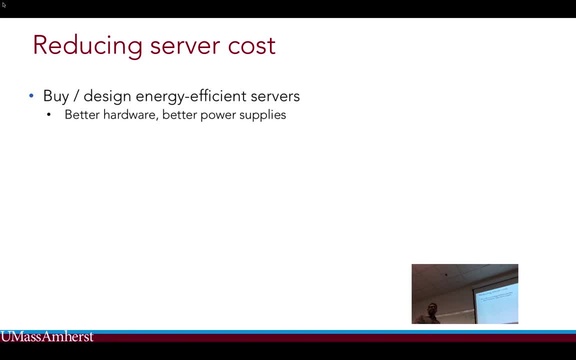 power supplies more efficient, power supplies which convert the AC power into DC to power all your machines. So you can go for a better power supply And this is non-intuitive, So you can actually use DC power and it can be more efficient than. 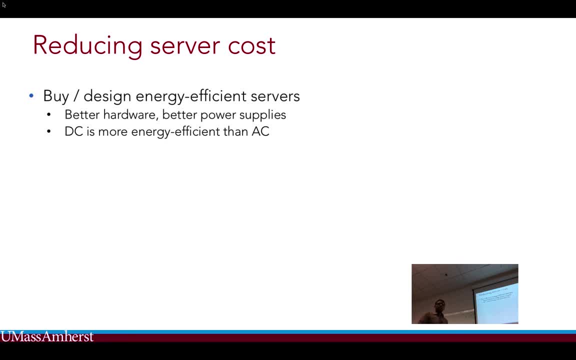 air and AC power. So from power electronics literature we know that AC power can be transmitted for long distances without loss. But the same cannot be true in case of data centers, because there are lot of conversions happening from right, from solar panels producing that power to step-down transformers- There's a lot of energy conversions that is happening. 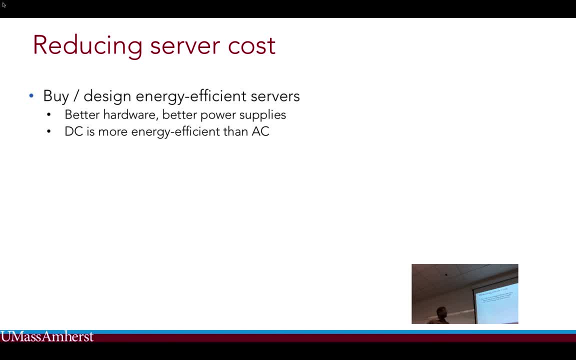 all along the line. So one line of research talks about directly using DC power So that apparently can save energy And you can obviously manage your servers better. intelligent power management policies turn off servers when not in use And of course you can pack many applications that are running on different. 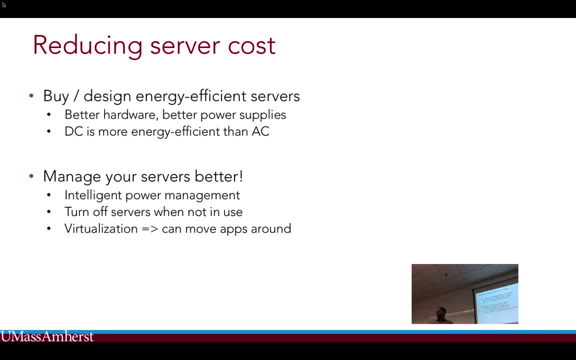 servers into one server through virtualization. So instead of ten different servers running applications which are not having high utilization, you can combine them and house it in the same machine And through virtualization you can actually fool the app by saying that, okay, it has its own dedicated resources like memory. 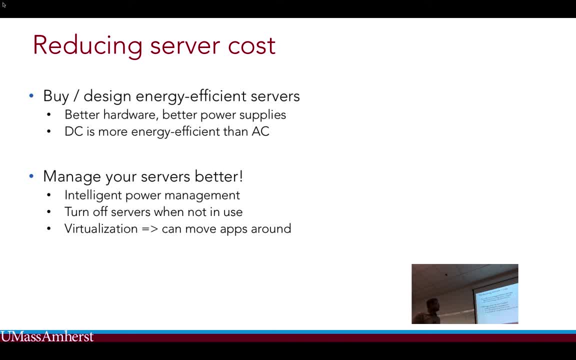 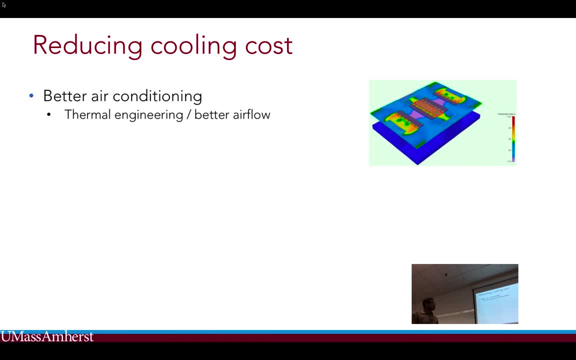 CPU cycles, etc. Reducing cooling costs. So one thing is doing better thermal engineering, better air flow- I think mechanical engineers are better suited to do that- And, of course, move to cooler regions, as I said. So you get free air from outside, which 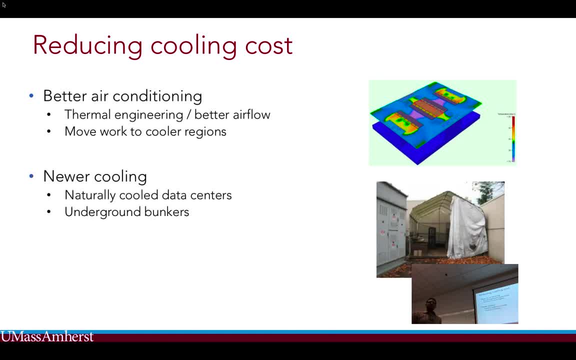 is cool. And of course you can naturally cool the data centers. And there is also another data center in Switzerland which uses geothermal energy for cooling, So they use subterranean cold water to actually cool the data center. So again, some innovative techniques which can 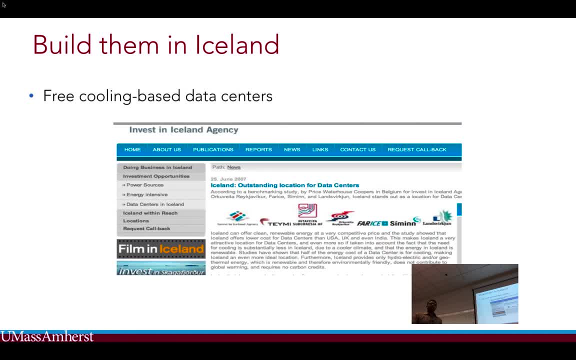 be used, And one solution is, of course, to build data center in Iceland. So there are many other considerations. So you don't- you may not always want this, because some applications are latency sensitive, So you don't want to experience the latency of pinging. 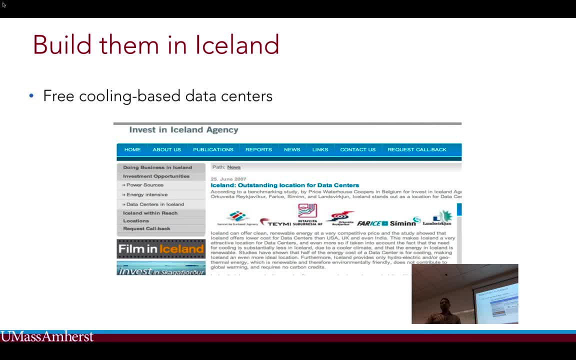 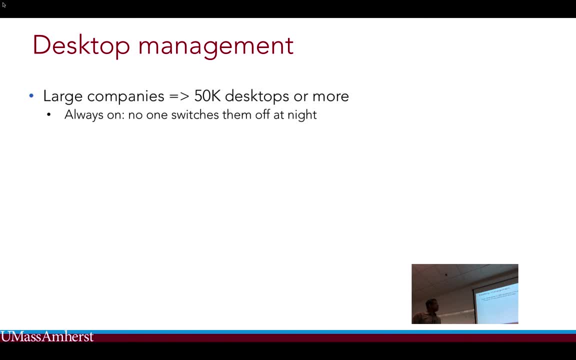 a server in Iceland and then back. So it may not be always possible for all applications, but for some applications obviously a promising solution. Now there are other strategies to reduce power consumption in corporations. That is through desktop management. So large companies have, say, around 50K desktops. They're always on. 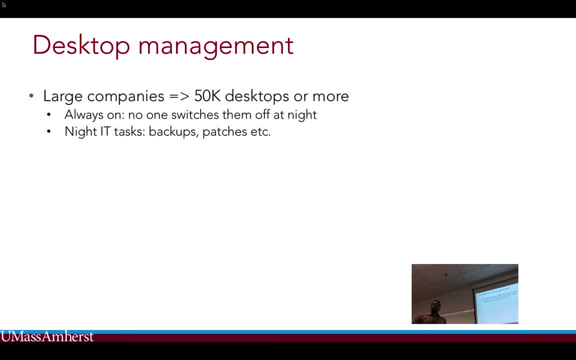 And many times IT tasks such as backup, security, virus scanning happen, So there are a lot of tests in the night, So you need to keep your desktops on throughout the day. Not ideal. Now, there can be better desktop policies, such as automatic sleep policies, And there was. 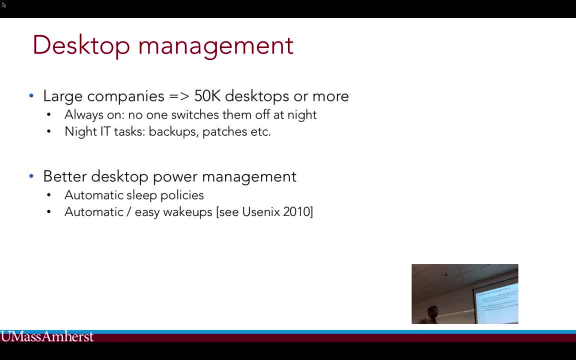 this work done in USENIC conference in 2010, where they make sure that there is a policy which ensures that there is easy wake up and user doesn't experience any distress, in the sense some security patch not being installed, So they make automatic wakeups- easy wakeups- possible so that you don't miss any security. 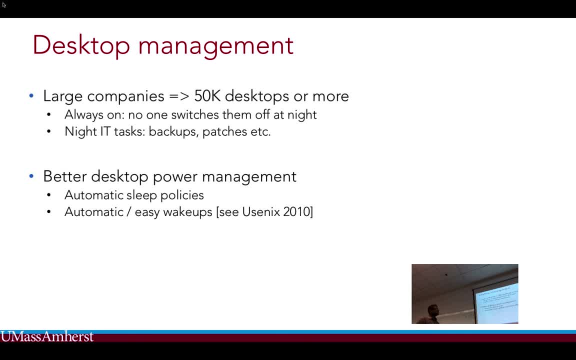 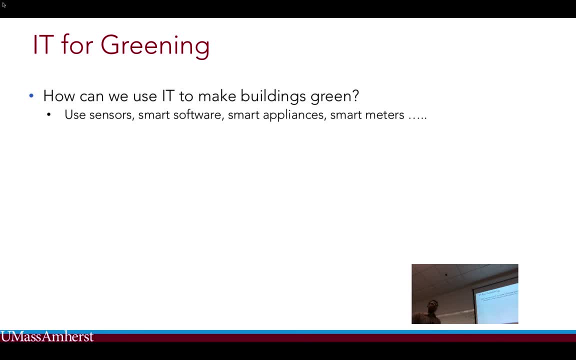 wakeups, security patches, but at the same time, you conserve energy. Now let's focus towards IT for greening. How can we use these sensor networks that we have seen or heard about in this lecture to improve the management of a building? How to make 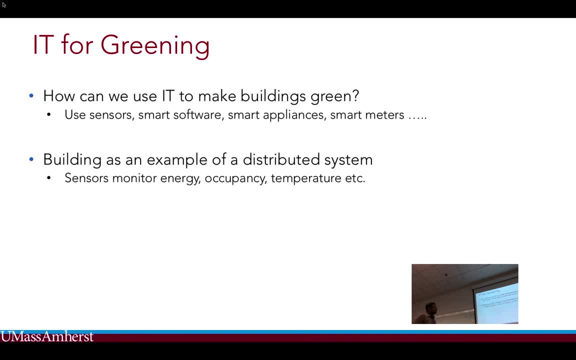 it more green. So one can think of building as a distributed system. It has hundreds of. a building like this might have hundreds of thousands of sensors. They monitor energy, occupancy, temperature And they analyze data in the sense. so there are these control strategies of when the lights should turn on when someone walks in And 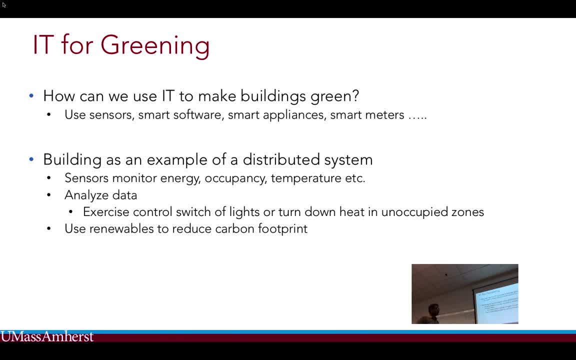 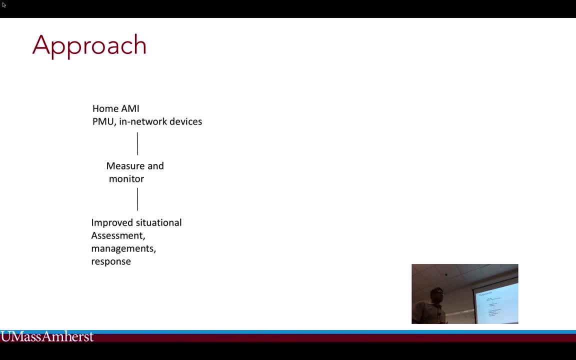 also one can use renewable energy to reduce the carbon footprint. So we can look at IT for greening at different levels. 1. One of the most important things is to look at measurement and monitoring. So most of the residential buildings in US come with what's called as a smart meter, which 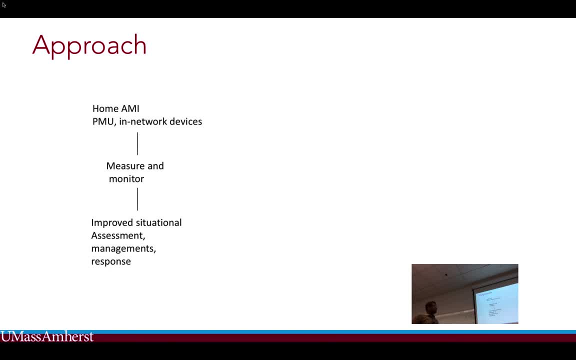 records the energy of a whole house. Similarly, there are other measurement entities which measure different aspects of a building And they have different application in terms of faster handling of outages. So through smart meters, the utility can know that. okay, This house is experiencing an outage. 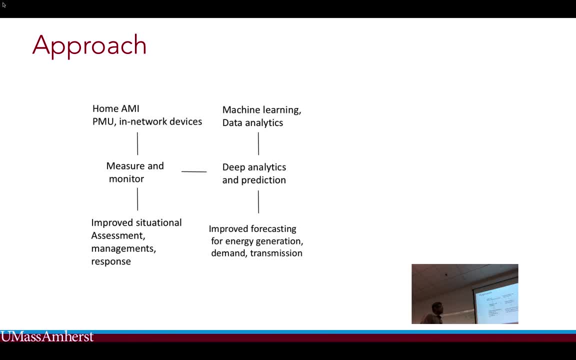 Send an engineer to fix it. Another aspect in which IT can bring greening is to provide analytics on the data that is generated. in this stage, You can do forecasting of energy and make sure that the energy supply demand is maintained in a grid. Many countries experience blackouts because of the supply demand being not matched. 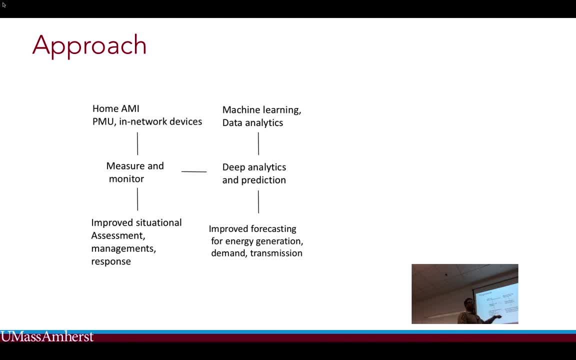 2. Using IoT deployments can actually improve the condition significantly, and employing machine learning techniques to predict energy usage in the future. And obviously, finally, you also want to control things. So many washing machines are coming up with ways in which they can directly talk to the. 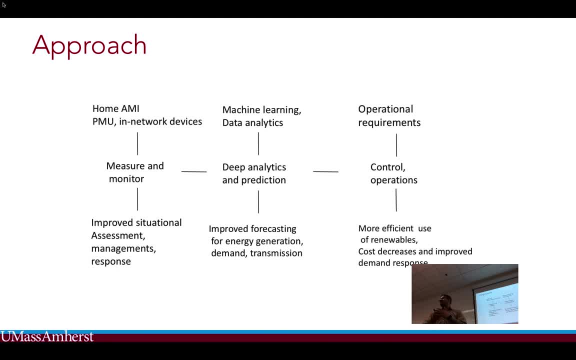 utilities, Get the price of electricity at that point in time And essentially delay there. 3. If you want to reduce the cost of energy use, you can do that by using a smart meter. So this particular technology is called demand response, where based on electricity prices. 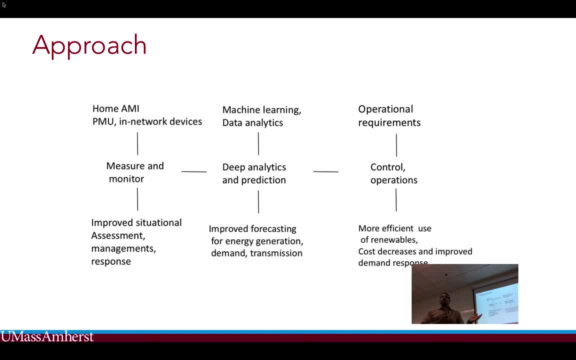 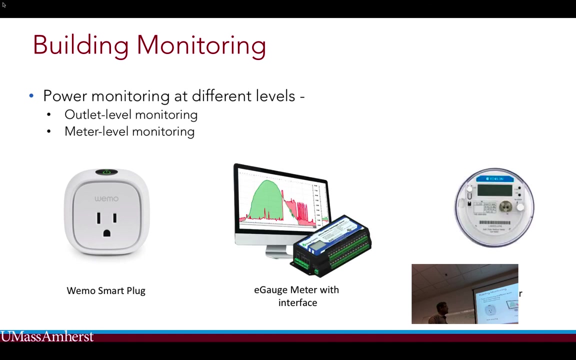 you shift your load, You shift your energy usage to non-peak hours of energy use. So in many countries the cost of energy is actually dependent on the time of use. So these kind of strategies can actually elevate the problem of peak demand. And building monitoring I have already discussed can be done at different levels. 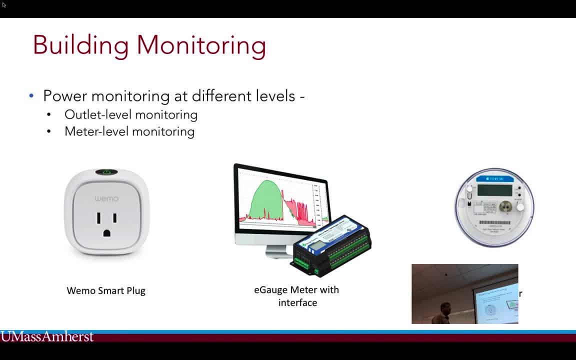 This is a plug meter which records energy usage at an outlet level. E-gauge is an energy meter for a whole house. It's actually a full Linux box and it can actually give you some cool dashboards to look at your energy consumption of your solar panels, your energy consumption. 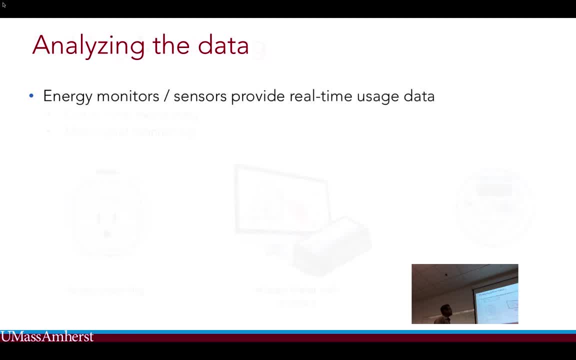 And, of course, there are smart meters that are installed all across the US 4.. Now, how do you go about analyzing the data? One is so: each building- actually each large building- has something called as a building monitoring system, And this actually takes information from different sensors to control the HVAC at different parts. 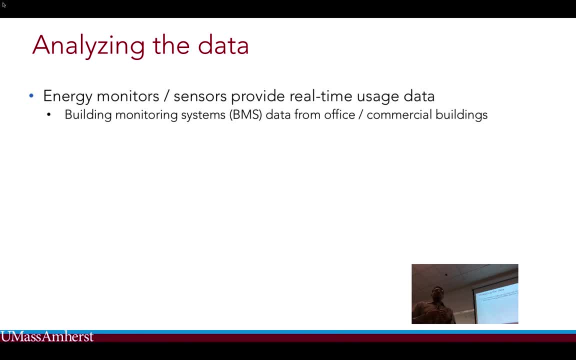 of the building recording the human doing people counting. so most of the cameras that you see in the campus Are employed with people counting sensors. So simple computer vision can be employed to see how many people are walking into the building, going out of the building. 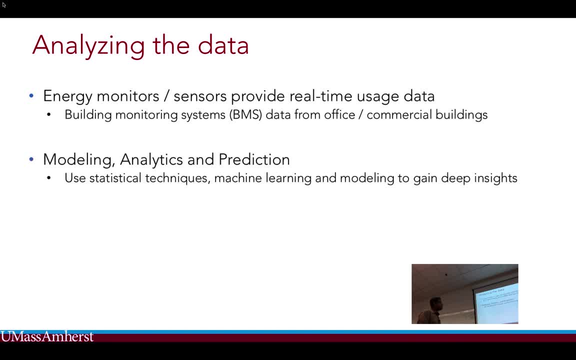 That can be insightful in controlling the HVAC And, of course, modeling, analytics and prediction. So you can use machine learning techniques to answer several questions. One is: which house has inefficient furnaces, heaters, dryers, or are you wasting a lot? 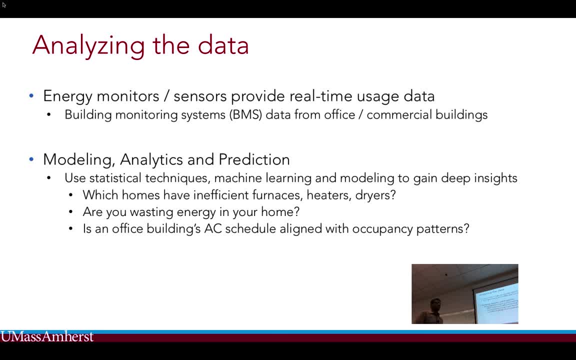 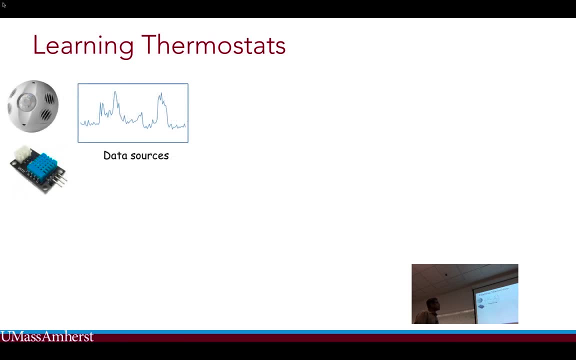 of energy in your house? And is an office building AC aligned with the occupancy pattern? And when will the aggregate load or transmission load peak? So these kind of prediction type questions can be answered by employing machine learning techniques. So a NEST thermostat will essentially look at a temperature, humidity sensor and an 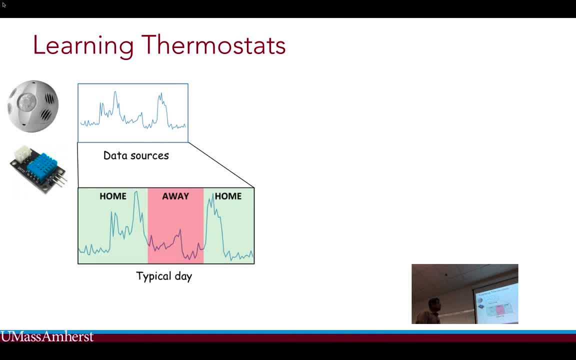 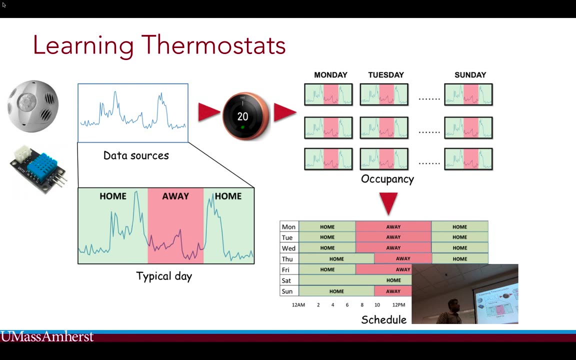 occupancy sensor to label the data as a person being occupied or a person who is not being occupied or away from the house, And this being repeated over several days, one can automatically learn a schedule- a seven day schedule- for a person. So NEST is increasingly using more and more advanced techniques to come up with faster 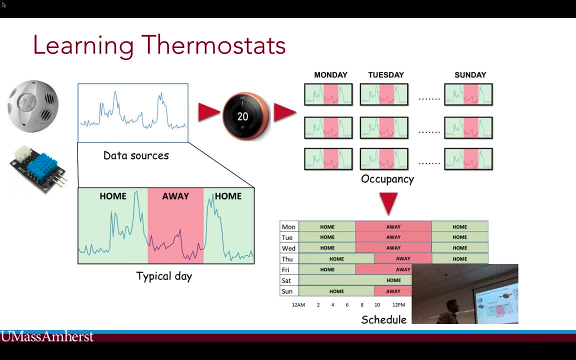 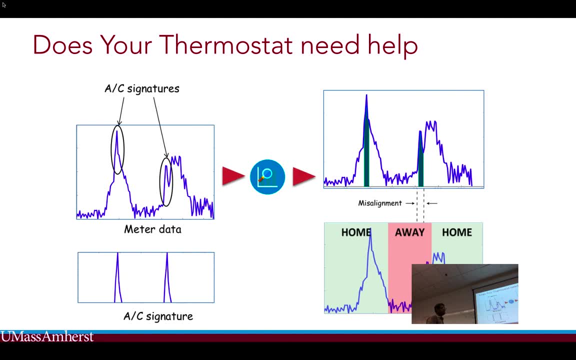 conversions to a set schedule. Similarly, it can identify any misalignment in AC usage. So, for example, here There is an AC signature which is identified and this misalignment can be used in the future to possibly shift the occupancy. make sure that the AC is never on when you are not in. 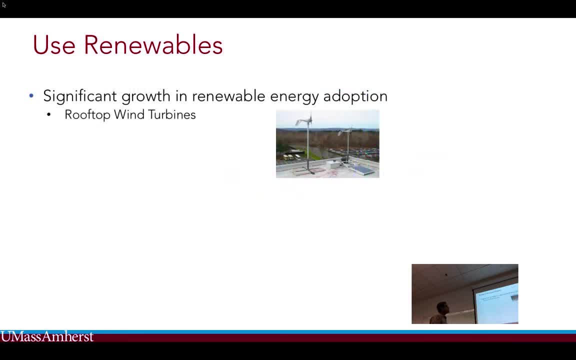 the house. So one way to handle or reducing our carbon footprint is by incorporating more renewables in our energy usage. There is significant growth in solar energy In US. in the last six years the solar deployment has increased from 2.3 gigawatts to 40 gigawatts. 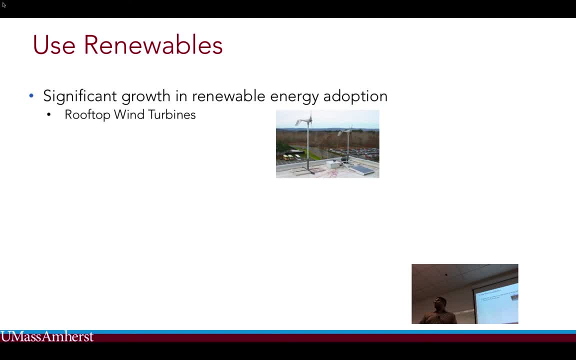 In countries like China and India. in the last year the solar deployments have doubled, So it's increasing all over the world. They can be in different forms, like rooftop wind turbines, which are not necessarily popular all across the world, but everybody knows solar PV installations, solar thermal, for 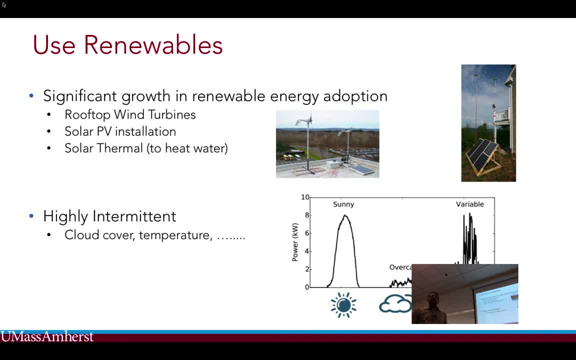 water heating. The problem with renewable energy is the intermittent nature, So photovoltaic panels are essentially nothing but p-n junction diodes. And the problem with p-n junction diode is they are sensitive to temperature And with temperature the resistance of the p-n junction increases, reducing the efficiency. 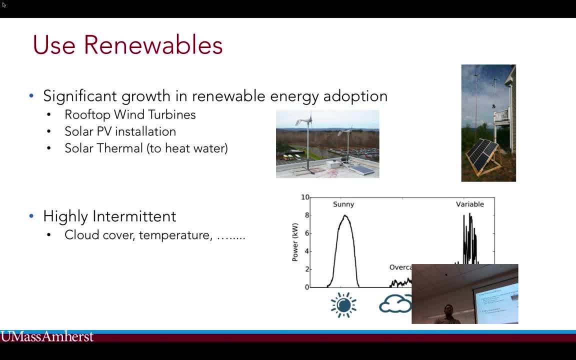 of the solar panels. Another problem is obviously with cloud cover, dust, snow. the amount of photons that are falling on the panel itself is reducing, So we have to be careful. Because of all these dynamic factors, solar energy is not necessarily highly predictable. 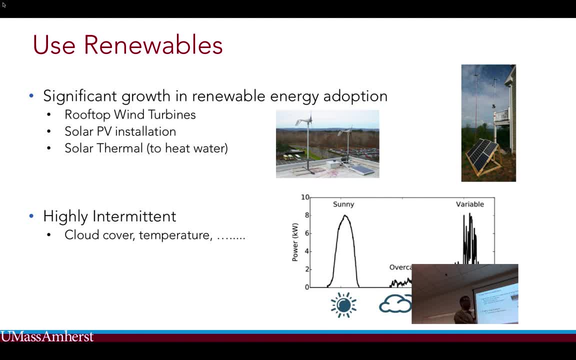 So in a very clear day, you will see this nice sinusoidal curve of energy that is generated using solar energy, And on an overcast day, you see something like this: very less power being generated. And on a scattered, cloudy day, you see that there are large gyrations in the amount of 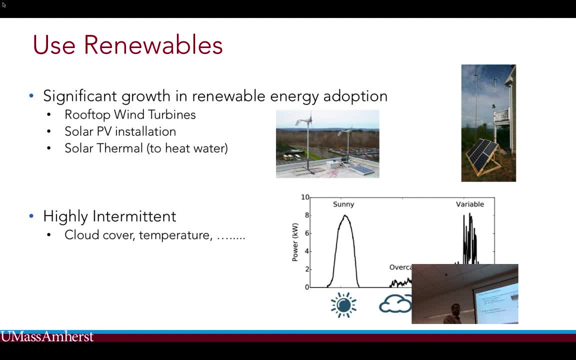 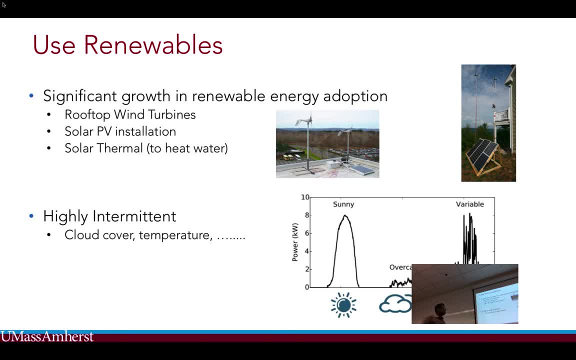 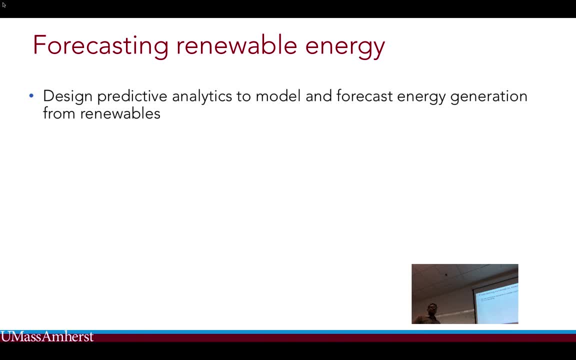 This can happen every week, such variations. So one problem is forecasting the renewable energy so that you can use this insight and leverage solar energy when it's being generated. So one can use machine learning models and weather forecasts to actually predict energy from solar or wind turbines. 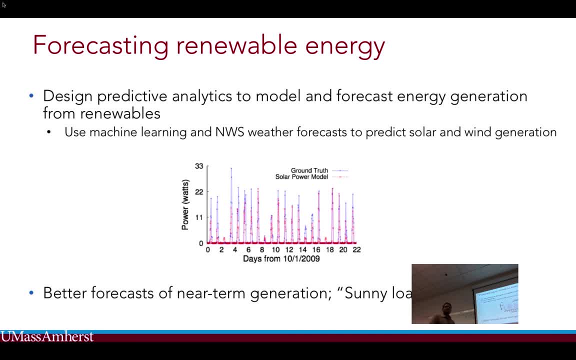 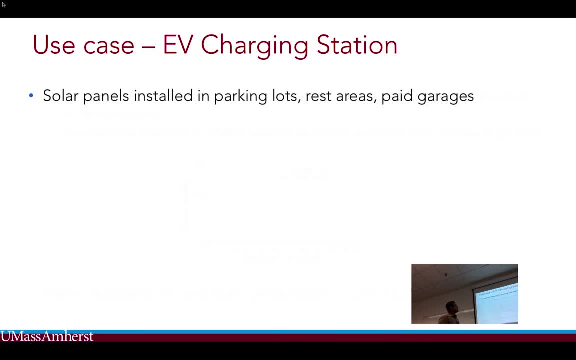 And these forecasts can be used for near-term generation And we can schedule some of the loads based on the solar energy being generated. So there are several use cases. One use case is to have an EV charging station. So in our university itself we have these parking lots with solar panels mounted on. 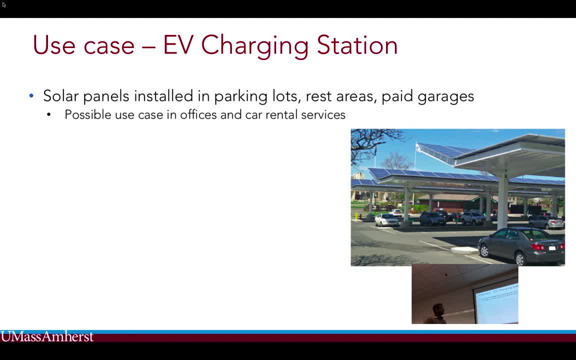 them. Imagine a possible use case of offices or a car rental service like Zipcar. So in these places you can actually make some assumptions about what will be the arrival or the departure rate of different electric vehicles And you can leverage some accurate solar prediction. 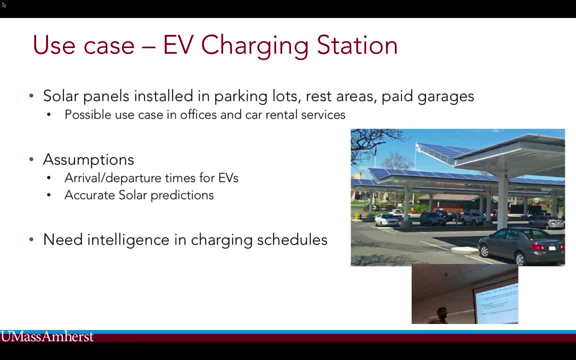 And based on these arrival departure rates one can have a very intelligent scheduling policy. So, for example, when you know the arrival departure of electric vehicles, this problem essentially translates to scheduling in a preemptive mode. So you can have a preemptive unit processor system. 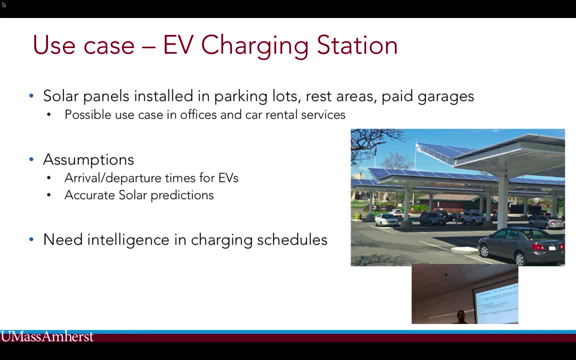 And the most optimal solution. there is earliest deadline first. So, as is the case with the jobs coming to a processor, if you know the arrival and departure timings of a job or, in case of jobs, you know the amount of resources that need to be dedicated. 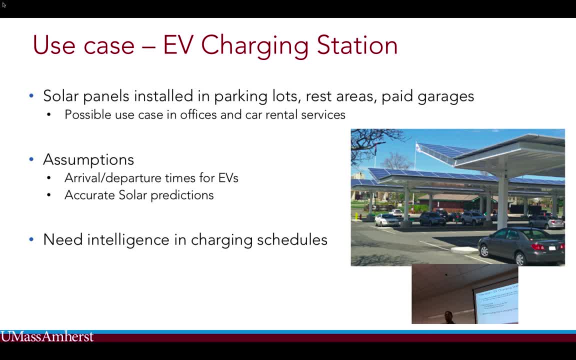 and when it needs to be completed. you can actually schedule them in an optimal way. Of course, not all these assumptions can be possible. So we can actually schedule them in an optimal way. Of course, not all these assumptions can be possible. 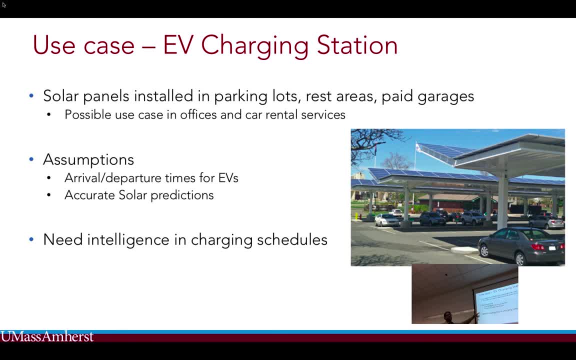 So when you can actually schedule them in an optimal way, you can actually schedule them in an optimal way. So when you can actually schedule them in an optimal way, you can actually schedule them in a real system. So maybe with different set of assumption you come up with a different algorithm, not 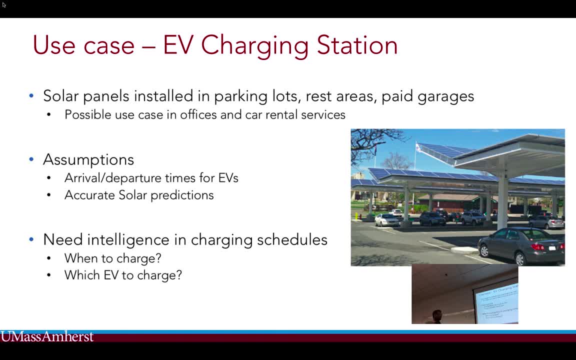 the earliest deadline first. And of course, these questions like when to charge, which EV to charge and how much to charge are not so straightforward. So imagine a case where there are two electric vehicles, So EV1 and EV2.. So EV1 has 90% battery charged and EV2 has 10% battery charge. 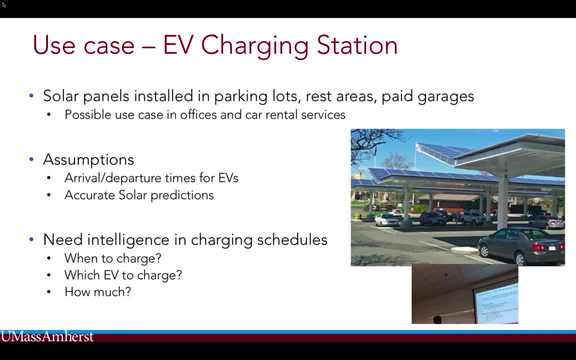 So obviously in this case, and if you have, say, X amount of energy, a fair strategy would be to just give X by 2 to this one, this EV, and X by 2 to this one. but it may not be fair Because this one already has 90% charge, so possibly you can give everything to EV2.. 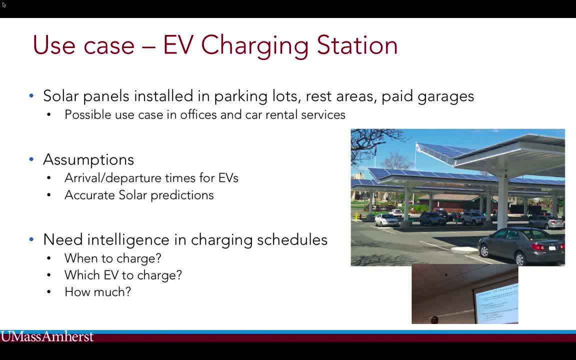 So I mean, this is a very simple scenario of just two EVs, the contention between just two EVs, But when we talk about dynamic arrival, departure timings and different assumptions or constraints in your system, designing a scheduling policy is extremely hard And in many cases, in fact most of the scheduling problems in this world, are NP complete. 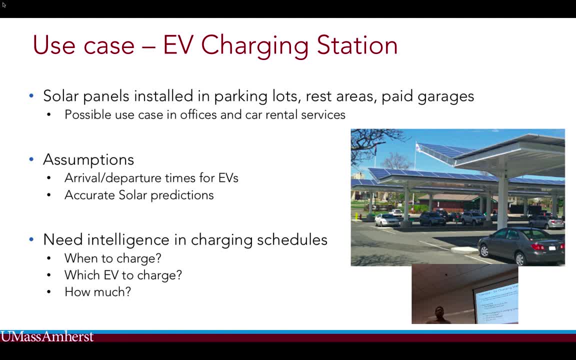 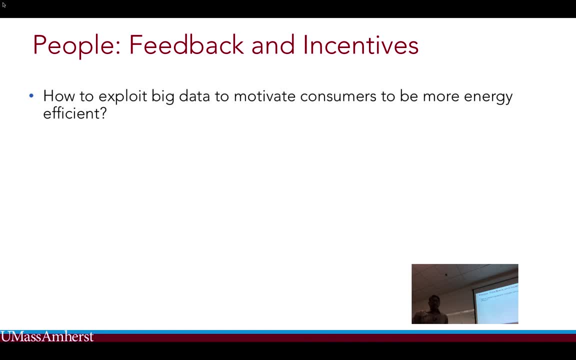 So So you need to come up with some kind of an approximation strategy to solve this problem, And obviously the most important challenge is to involve people in decision making, in the sense provide some kind of incentives to reduce energy usage. One way of doing it is to have immersive apps, provide a game in which you say that OK. 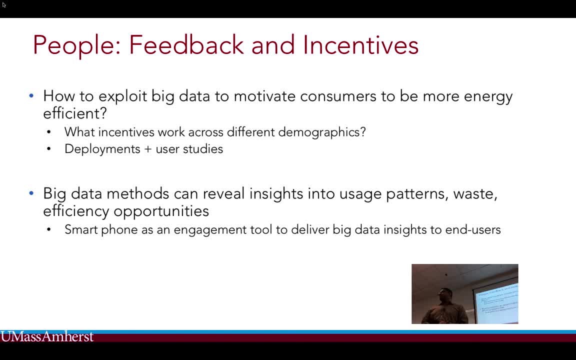 reduce your thermostat So you can set a set point by one degree and you will get some green points. Such experiments have been done in the past and have proved to improve and have resulted in improved energy efficiency or reduction in energy usage. And, of course, you can provide personalized feedback about your energy usage.